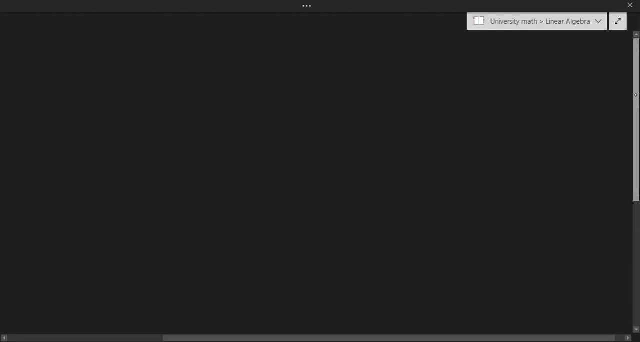 Hello and welcome to another video. So in this video we'll be talking about the concept of norm. So what is the norm of something? Well, if you ever took a course in physics or anything like that, you may have heard the term magnitude. Well, a norm is just a. 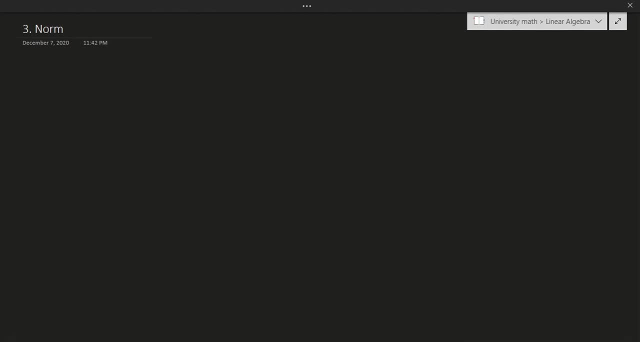 very fancy way of just saying the same thing. So, by definition, the norm is the magnitude of a vector. So more or less that's what it is. So let me just write that down. So the norm is essentially just the magnitude of a vector, And that is essentially what 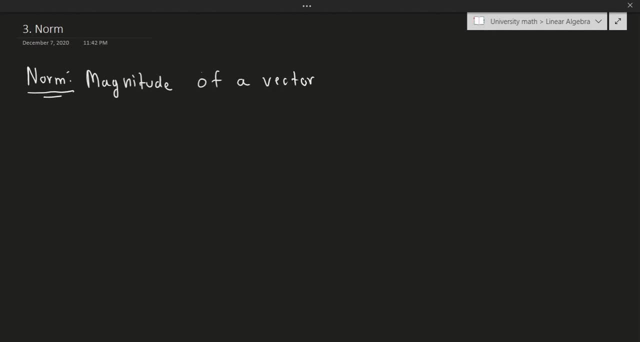 a norm is. Now, how do you calculate the magnitude of a vector? And before I go on, you can also say equivalently that the length of a vector is the same thing as a norm as well. These are both equivalents, These are both equivalents statements And they mean the exact same thing. So, as a result, 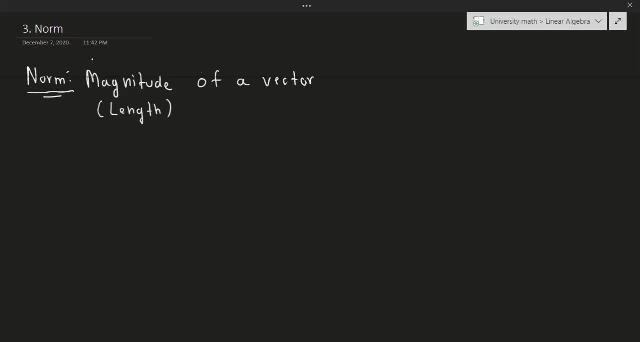 you can say these like: correspondingly: Okay, now that aside, how do you actually calculate the length of a vector or the norm of a vector? Okay, so suppose I give you a vector x composed of the components x1,, x2, and so on, all the way to xn. So this is. 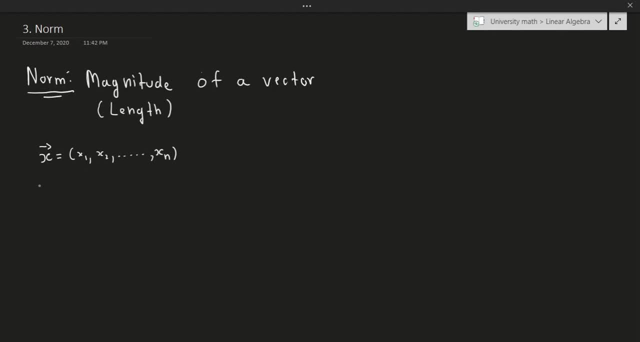 an rn, So the norm which is denoted by these double kind of bracket, these lines of some vector x which we enclose with these double kind of lines. So this is the definition of a norm. So, symbolically, this is how you write a norm. So the norm of a vector is equal. 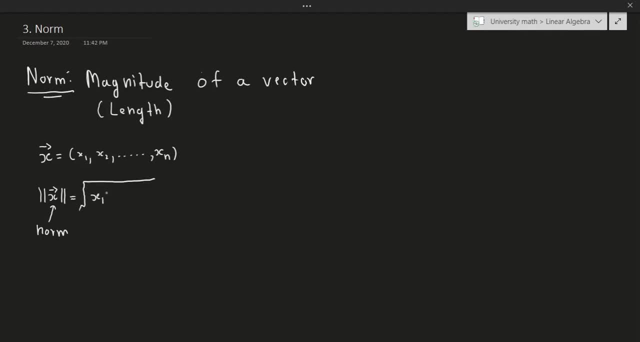 to the square root of x1 squared plus x2, squared plus dot, dot, dot. So we just squared each of the components All the way from x1 to xn And then we just simply take the square root of that. So this: 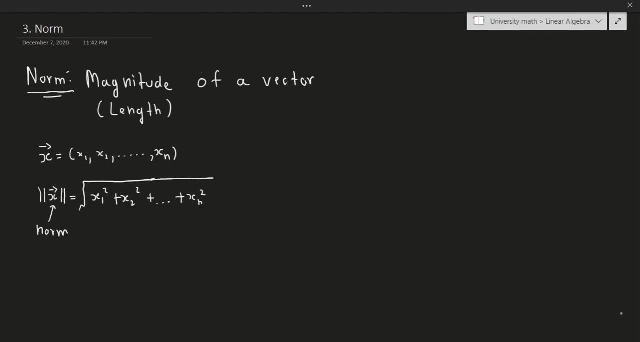 is how you calculate the norm of a vector. So that's all there is to it, to calculating norm. So there's nothing particularly challenging about this. Now, how do you, kind of you know, characterize this? So how? what are some properties of the norm? So let's go. 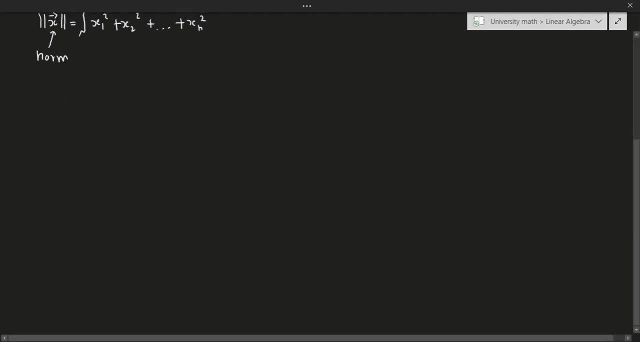 ahead and write down some properties. So some properties. OK, There isn't too many properties here. So the first one is that the norm of a vector is always bigger than or equal to zero. Induitively, that should make sense. The norm is the square. 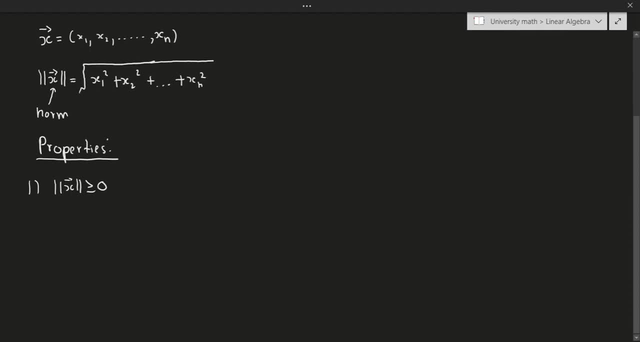 root of a bunch of components, and the square root of a number is always zero or bigger, in the real numbers at least. OK, So the second one: the norm of a vector is equal to zero if, and only if, the vector –. 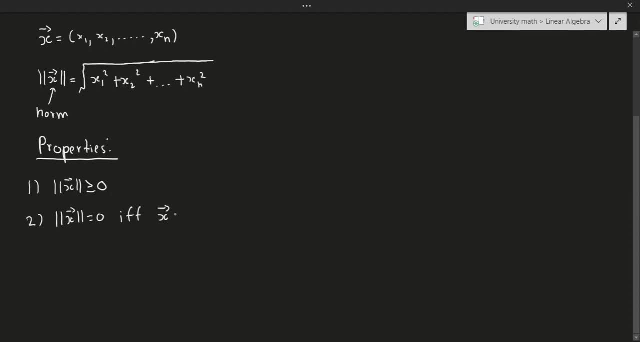 The answer is. The answer is …. vector itself is the zero vector And intuitively, this should again make sense. If even one of these vectors are non-zero, then the square root of something non-zero can never be equal to zero. That doesn't make sense, Even if, for example, if you had the square root of 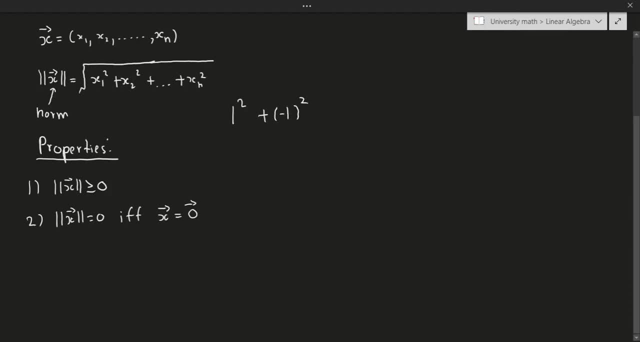 1 squared plus negative 1 squared, that still wouldn't be zero, because that's going to be 1 and that's going to be 1.. So the square root of this kind of mess is not going to be zero in any way. So, as a result, the norm of a vector can only be zero if the vector itself is a zero vector. 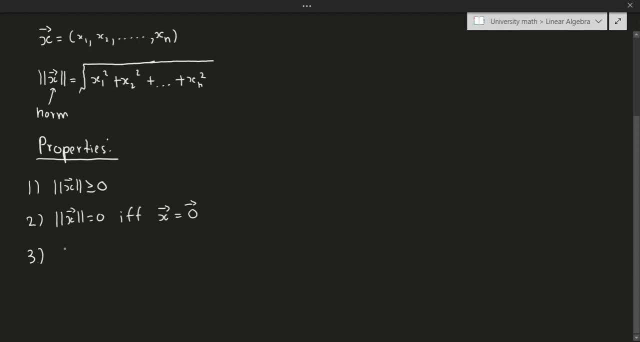 Okay. so the next one is suppose I have the norm of some scalar t multiplied by some vector x. This is equivalent to the magnitude or the absolute value of that vector, of that scalar. sorry times, the norm of that vector. Now I should probably make a small kind of note here. This is the absolute value of a scalar. 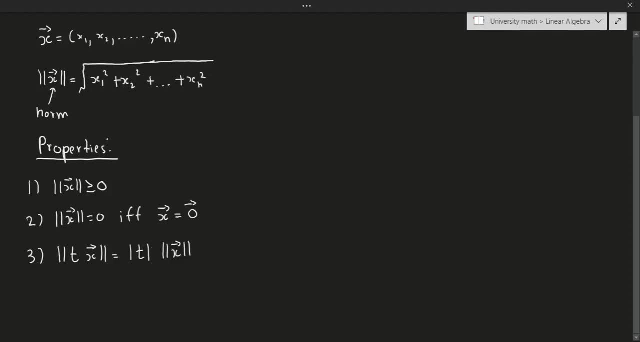 This is the norm of a vector. They're very similar, but there's some very slight differences in the terminology. Nevertheless, take a look here. I'm just saying that if I have a scalar, so if I have a scalar t, I can pull the scalar out and take the absolute value of it and then multiply it by the. 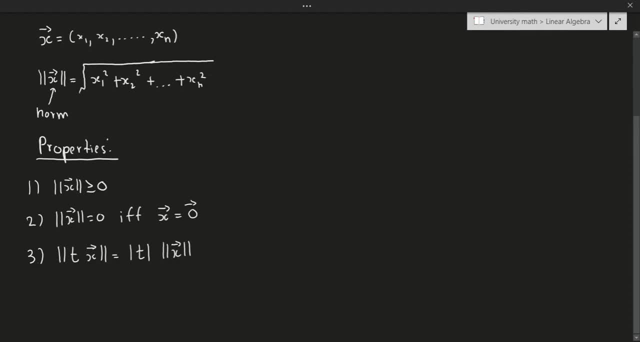 norm of the vector. So I can just pull out any kind of scalar from a norm of a vector, So I can. So in this situation t is a scalar. Okay, so the next one. technically I should- I shouldn't be using real numbers- So t. 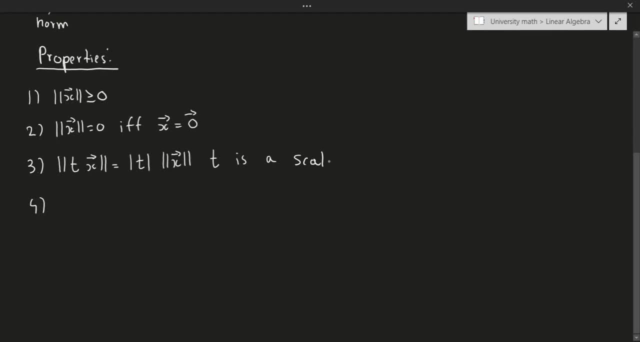 is a scalar. Let me just go ahead and write that down, Okay. the next one is a little bit of a unique situation. This one is the triangle inequality. This one says: if I have the norm of x plus y, this is always less than or equal to. 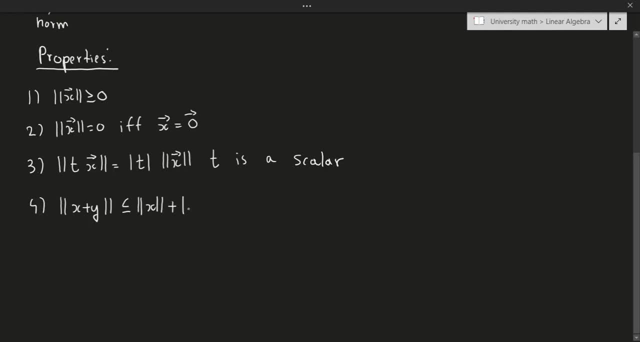 norm of x plus the norm of y. Now, the proof of why this works requires something called the Cauchy-Stewart's inequality, which is something I'm not going to be doing for a very long time. so I'm going to skip the proof of this inequality, but rest assured that 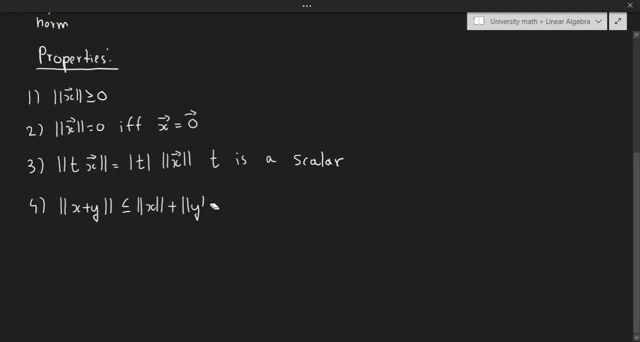 this is definitely something that's valid and intuitively should make sense, So let me just write that down. So this is known as the triangle inequality. Okay, and, as I said, I'll be skipping the proof of this, just because the analytical proof of this can be. 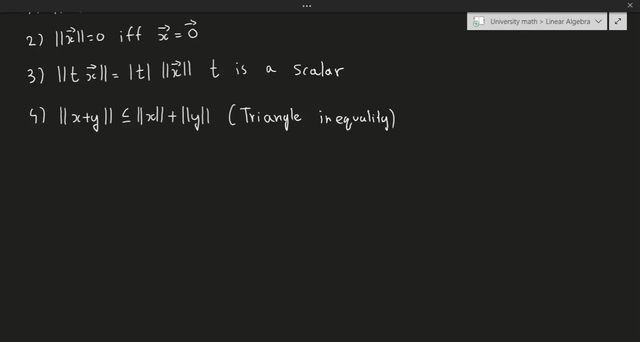 a little bit strange, so I'm not going to spend any kind of time talking about this. the proof of the triangle inequality. I'll do it later, but not right now. Okay, so the next one is the concept of a unit vector, So I'll just go ahead and write that down. 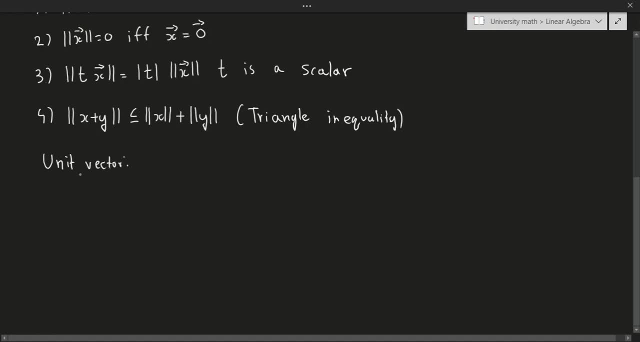 so a unit vector. Okay, so if I have some vector v, so v is say to be a unit vector to b and unit vector, which is what I'm writing a little bit. so unit vector if the magnitude of v is equal. 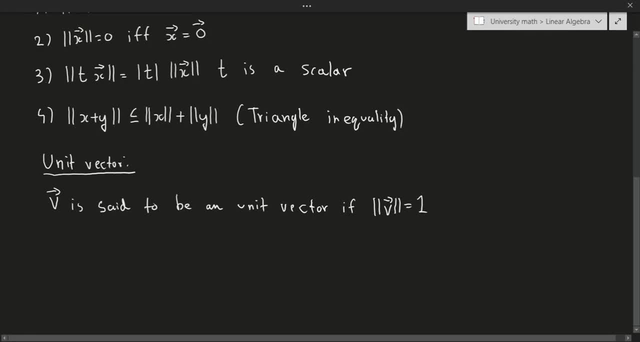 to 1.. So, basically, the norm of the vector is equal to 1.. So you'll see me interchanging the word magnitude and norm quite often They both mean the same thing, so I'll be interchanging the terminology whenever I feel like it. Okay, so let's keep going. So essentially what? 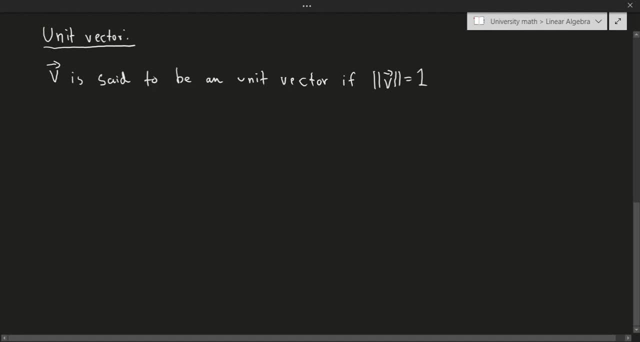 I'm saying is that if the vector is equal to 1, then the norm of the vector is equal to 1.. So essentially, what I'm saying is that if the vector is equal to 1, then the vector is equal to 1.. Now, even if the vector has a magnitude or norm of 1, we call it a. 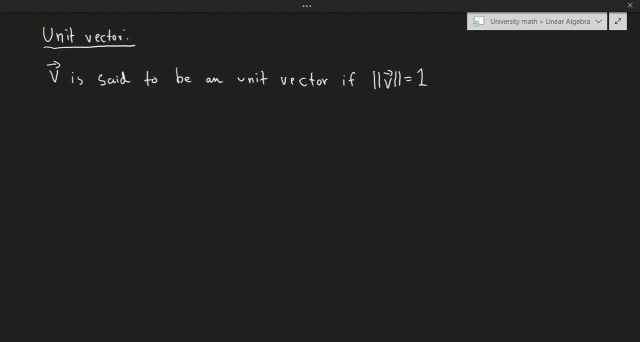 unit vector. The unit vector you could take over as sort of a tool to help us find the direction of a vector of sorts. but let's just go ahead and talk about that a bit later. So let's do a couple of very quick examples- and by I says a couple, I mean a little bit. 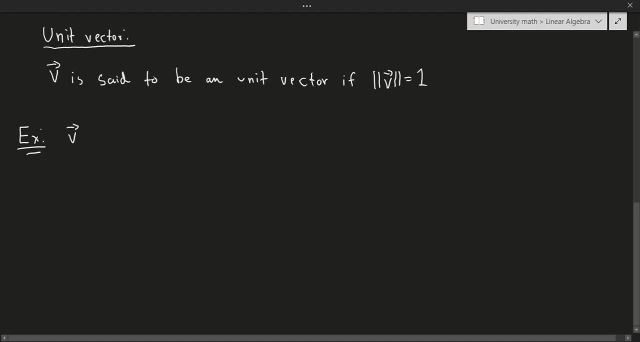 more than two. So suppose I have v is equal to minus 5,, 3, and 9.. So what is the norm? is the norm of v? Okay, well, that's, that's very simple. So in order to calculate the norm of the, 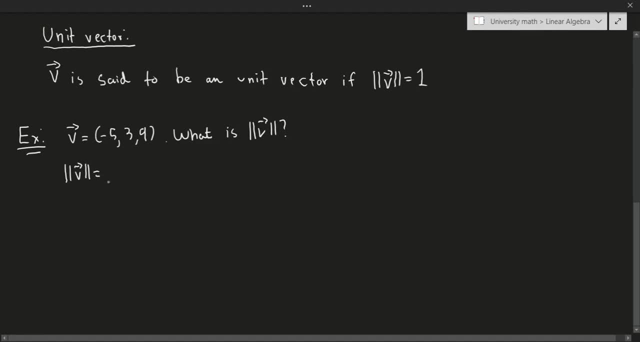 vector. I simply go ahead and take the square root of each of the components squared, So it'd be negative: five squared plus three squared plus nine squared. Okay, so if I go ahead and calculate this, this will give me a square root of 25 plus nine plus nine. So let's go ahead and 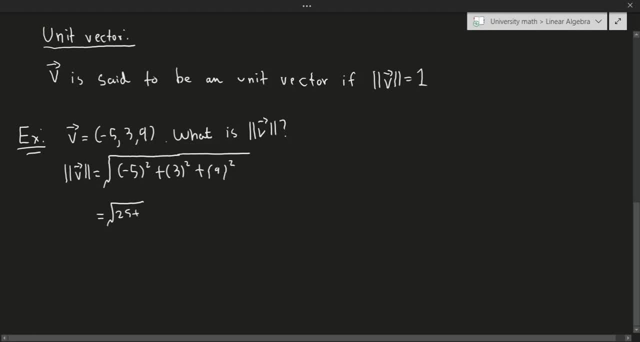 write that down. So 25 plus Oh, that's yet 25 plus nine plus 81.. Sorry, And so that's going to give me the square root of 25 plus 90, which is the same thing as the square root of 150.. And that. 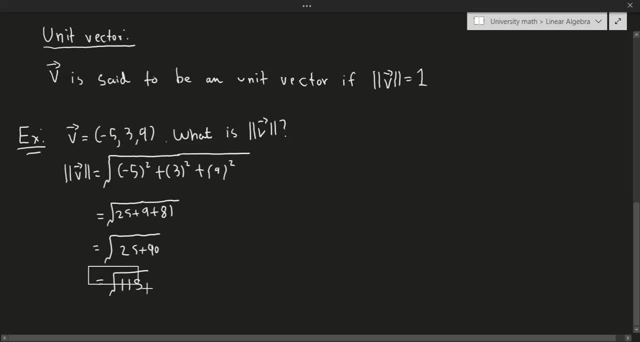 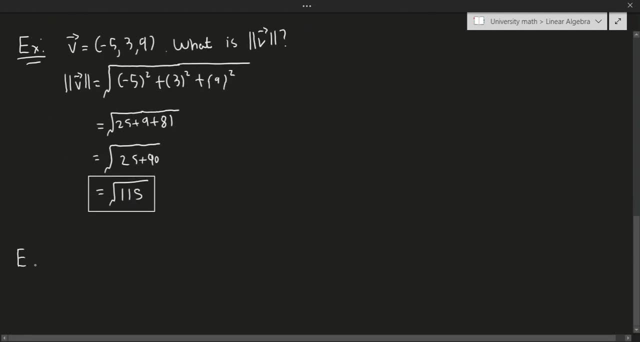 right, there is our final answer. So there's nothing too complicated about this, we just literally go ahead and plug it in. Okay, so let's go and calculate the next one. So this one is suppose we give you that suppose I give you rather, that j is equal to 010.. So, in this situation, well, the magnitude of j, So let me just 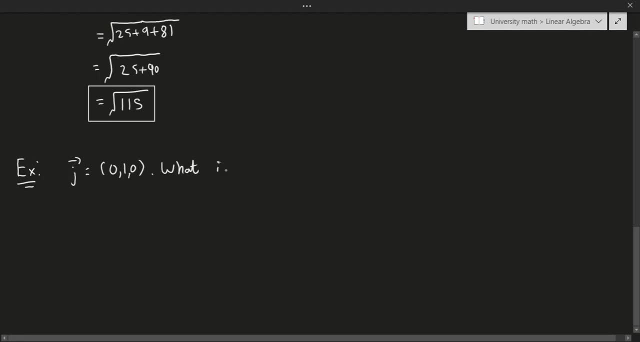 explicitly write this down. So what is the norm or the magnitude of j? Okay, So this is again pretty simple. So the magnitude of j is equal to the square root of zero squared plus one squared plus zero squared. Okay, but that's just equal to square root of one, But the square root of one is just one, So that's. 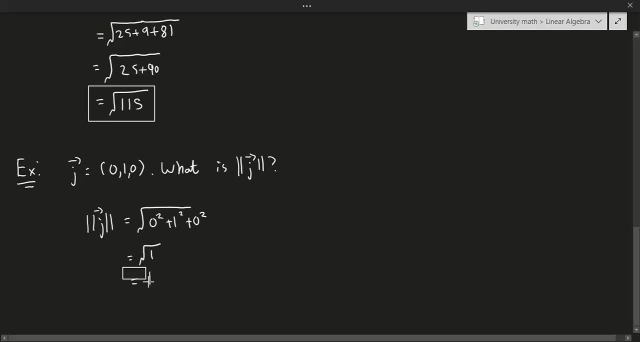 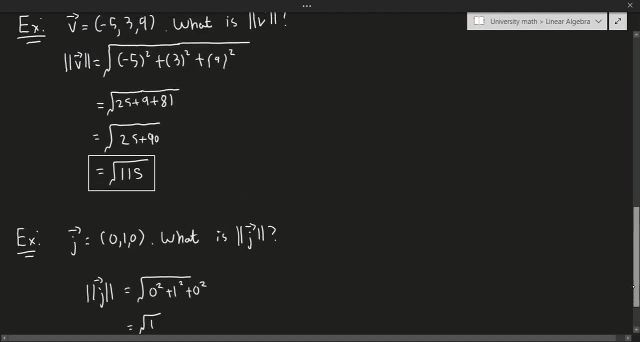 just our final answer. This is extremely straightforward And, as a side note, because the magnitude is one, this is a unit vector. because we define the unit vector to have a magnitude of one, that was given right there. Okay, let's talk about. 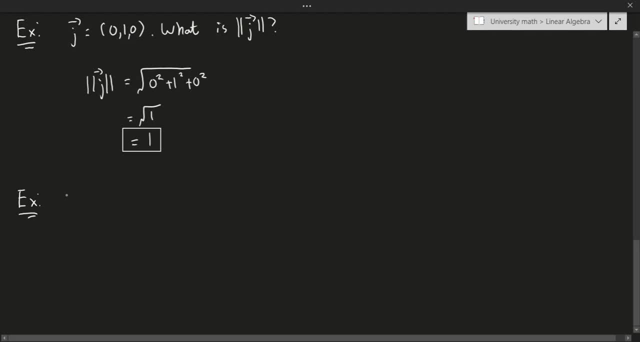 next one. Okay, so suppose I give you that w is equal to three comma minus four. So, in this situation, what is the norm of w? Okay, well, that's once again pretty straightforward. This time we don't have three. 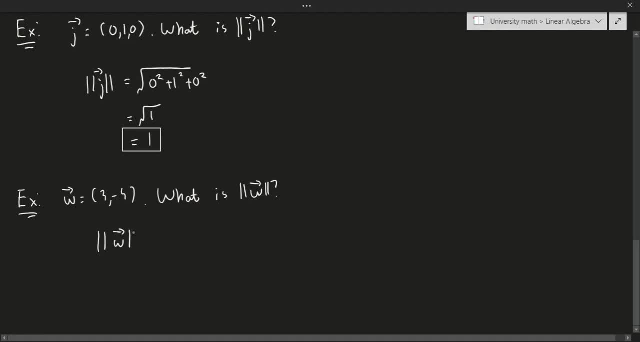 components. but that's okay. So in this situation, the norm of w is equal to the square root of three squared plus negative four squared. Well, that's the same thing as nine plus 16.. But that's just equal to 25.. So the square root of 25.. Well, that's just equal to five. So the norm of w is just equal to five, And that's all. There's nothing too complicated about this. 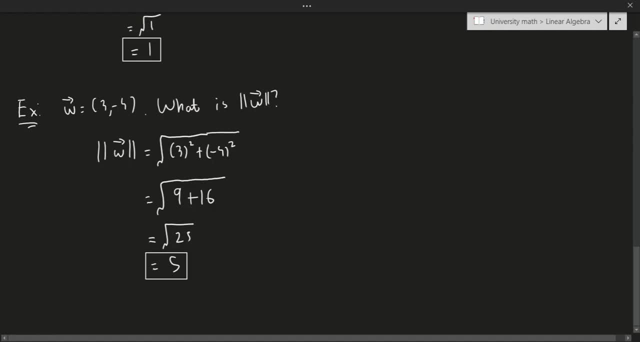 Okay, now the next thing we need to talk about is the concept of normalization. So let me just go ahead and write that down. So normalization- So you might be thinking you are missing normalization, meaning that you might be converting a vector into some kind of different situation, And 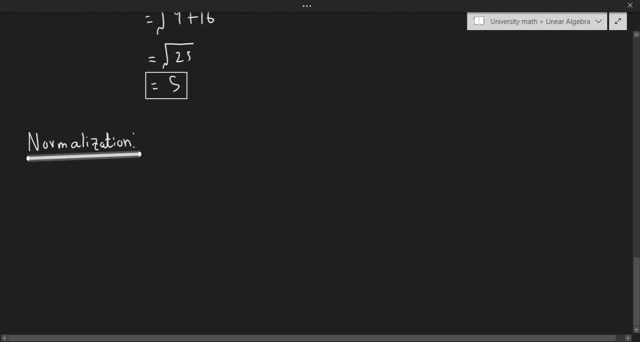 you are right. So what's going on here is that you're essentially taking a vector and forcing it to make it to become a unit vector. So essentially I'm allowed to take any vector and convert to a unit vector by just dividing by its norm or its magnitude. 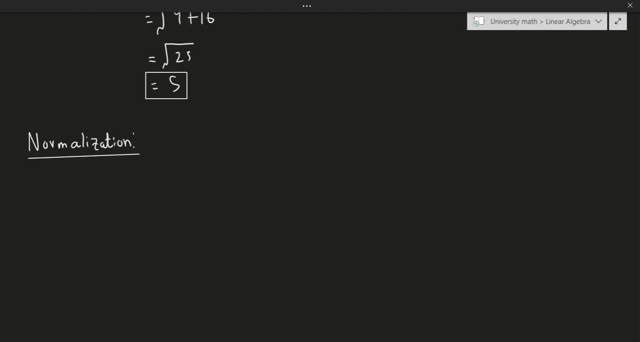 So in other words, for some vector v we can convert v. So for some vector v we can convert v to a unit vector which we're going to call u. So I know they look similar, so we'll just fix that. 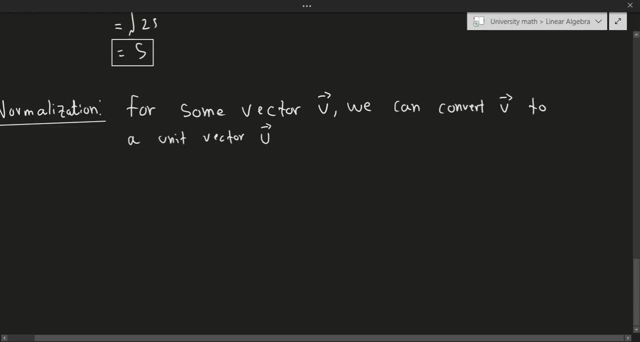 So for some vector v, we can convert the vector v to a unit vector u by dividing So v by the norm of v. So we can divide v by the norm of v, And that's all. So what am I saying here? 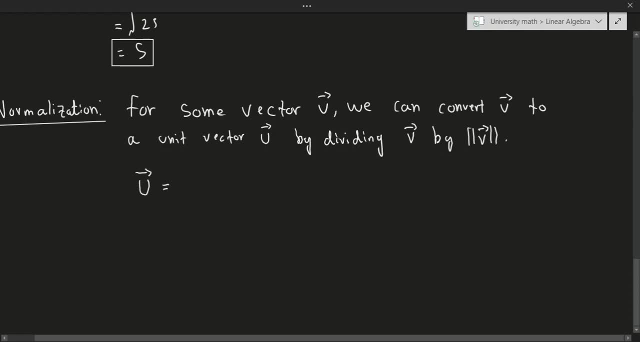 We're saying that some unit vector u is equal to v divided by the magnitude of v. So, as I just said, if I take v and divide it by it's magnitude or norm, we get some unit vector Okay. So let's go ahead and do an example of this. 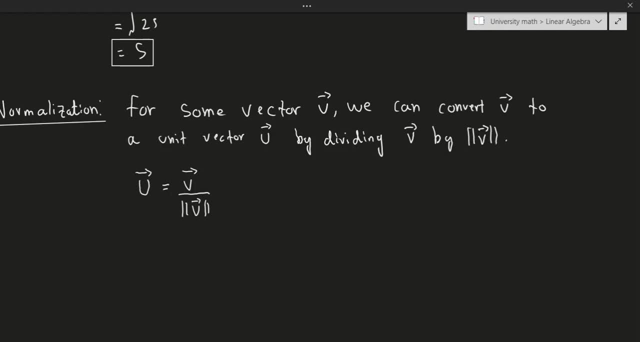 So let me just go ahead and take a look at my example right here. So essentially what I'm saying is that, given some vector v, I'm allowed to take any vector. It doesn't matter what kind of vector I have If I take any vector and divide it by. 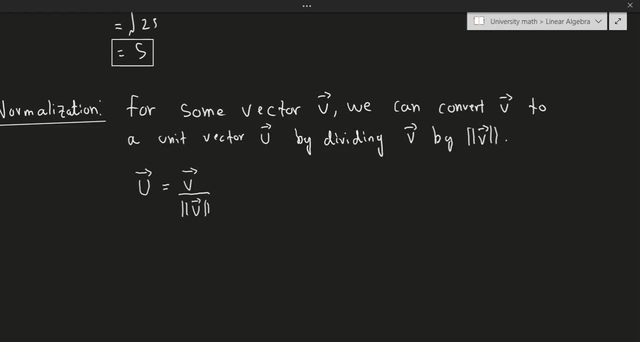 it's magnitude, I will always get a unit vector. So let's take a look at an example of this. Okay, Let's just scroll down. Okay, So let's take this example. Suppose I give you v is equal to 3, negative 1, and minus 2.. 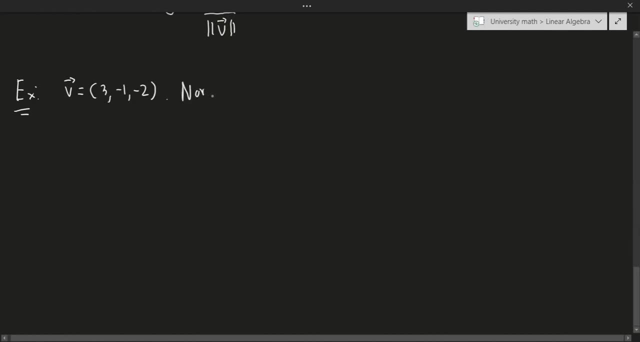 So what I'm saying here is normalize v. So this might seem a little bit of a very ill-defined because it's so short, but I promise you it's not. So let's just go ahead and calculate the magnitude, because we need that. 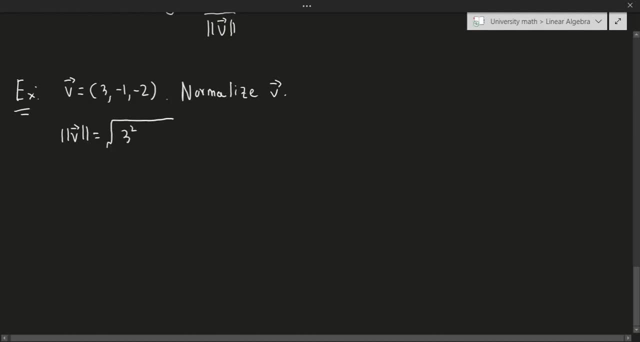 So the magnitude of v in this situation is equal to 3 squared plus negative, 1 squared plus 2 squared. So if we go ahead and do that, let me just fix my writing a little bit, Okay. So if we go ahead and do that, we get 9 plus 10, that's 10.. 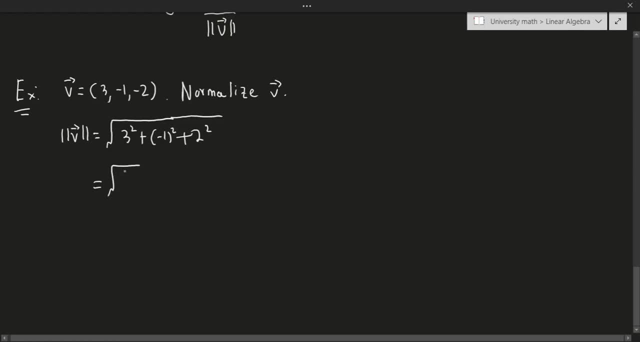 Then that's: let's see, we get 14.. So we get square root of 14 as a result, So a unit vector, so the unit vector that corresponds to this vector, v, would be equal to v divided by its magnitude. 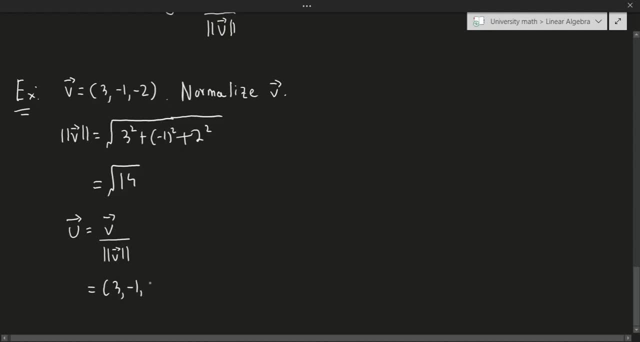 Okay, So that means we get 3, negative 1, and negative 2.. And then we would simply divide this by its magnitude, which is the square root of 14.. So all we do here is we divide each of the components by the square root of 14.. 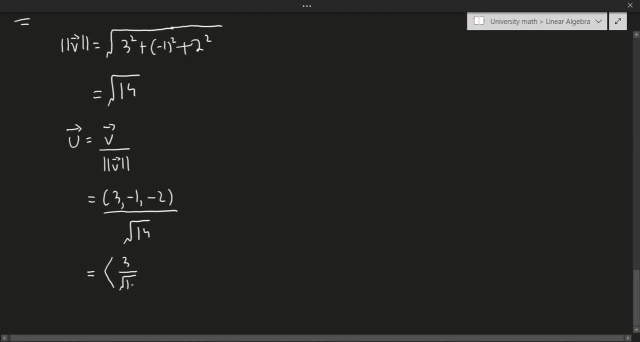 So this gives us 3 over the square root of 14, negative 1 over the square root of 14, and minus 2 over the square root of 14.. And this, right there, is our unit vector. You'll see that I use kind of different kinds of brackets to do this. 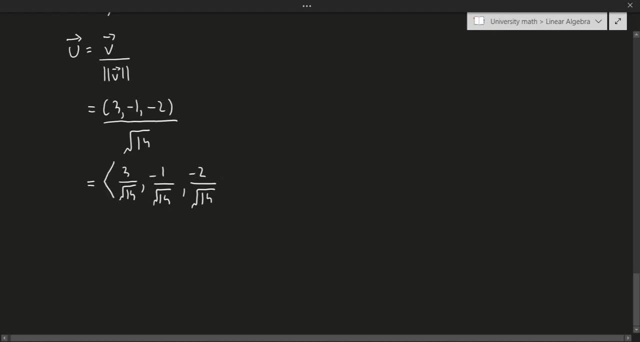 Typically in vectors, we usually use a set of straight brackets, kind of like that, But this isn't strictly necessary. Now I claim that this is a unit vector. Well, how do I know that? Well, we can use. we can just go ahead and verify this for ourselves. 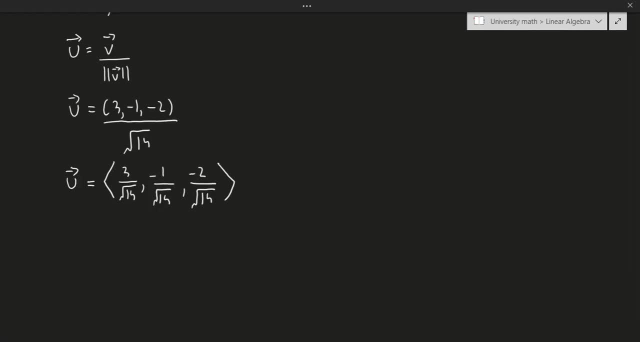 But I promise you that if you take the magnitude of this vector, you will get 1.. So let's just go ahead and check that. So if I take the magnitude of this vector, I claim that I'll get a unit vector. So the magnitude should be 1.. 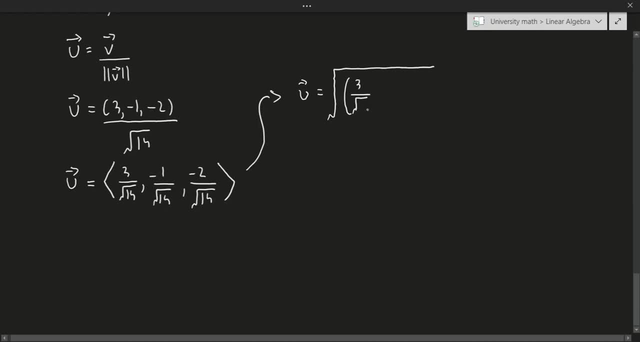 Okay, So 3 over the square root of 14 squared, plus negative 1 over the square root of 14 squared, plus negative 2 over the square root of 14 squared. Okay, So this gives us- let's see that gives us 9 over 14, plus 1 over 14,, plus 4 over 14.. 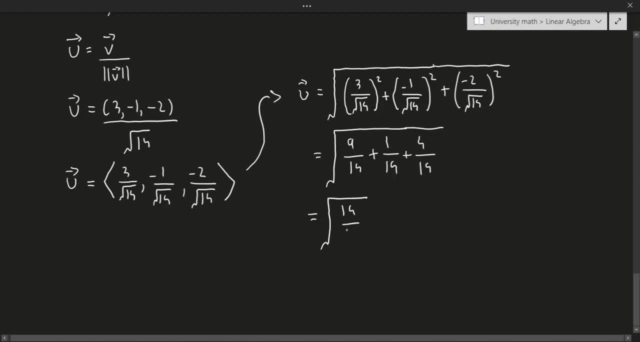 And that gives us the square root of 14 over 14.. But that's just the square root of 1, which by definition is 1.. So this is indeed the correct procedure to normalize any vector I want Into a unit vector. 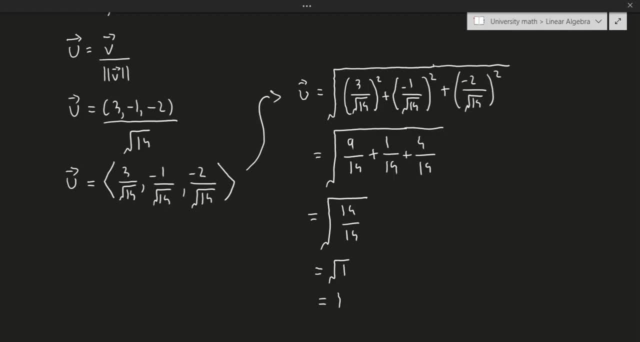 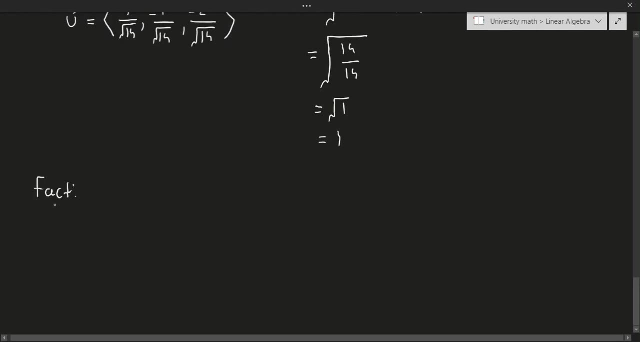 So that's great. Okay, Now let's talk about a new kind of concept right here. It is always true, and this is a fact, So let me just go ahead and write this down: Any non-zero vector. So let me just clean a few things up. 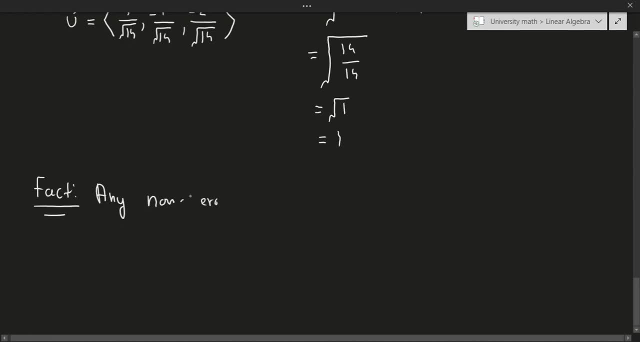 So any non-zero vector- Here we go- Is parallel to two unit vectors, And remember that this is the symbol for parallel- Is parallel to two unit vectors. So, essentially, what I'm saying is the following: So let me just go ahead and make sure I'm doing everything. 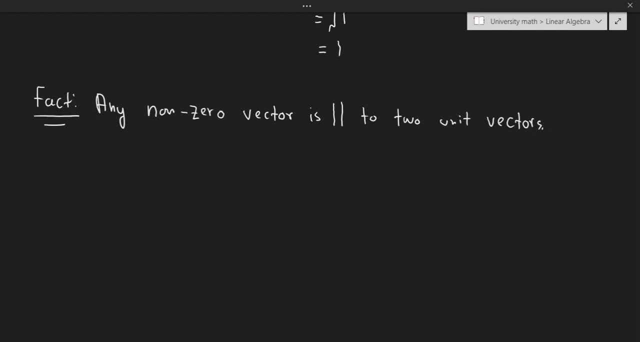 correctly. Yeah, pretty good. Okay, so any non zero vectors is parallel to parallel to two vectors. So what I'm saying here is essentially that if I have some non zero vector, it's parallel to one vector which goes in the same direction as the original vector And it's 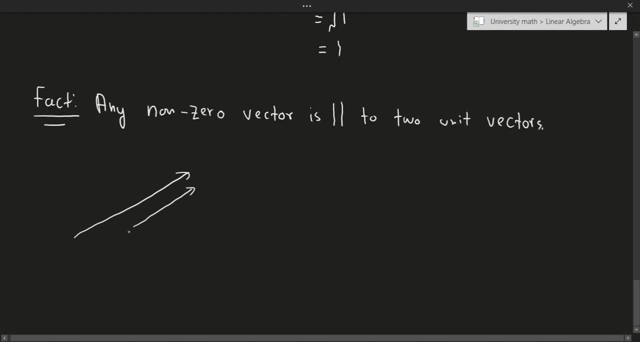 parallel to another vector which goes in the same direction, which goes in the direction, but it's opposite to this original vector. So what do I mean by that? That might seem a little confusing, So let me just kind of demonstrate this with an example. So suppose I give you the same vector. 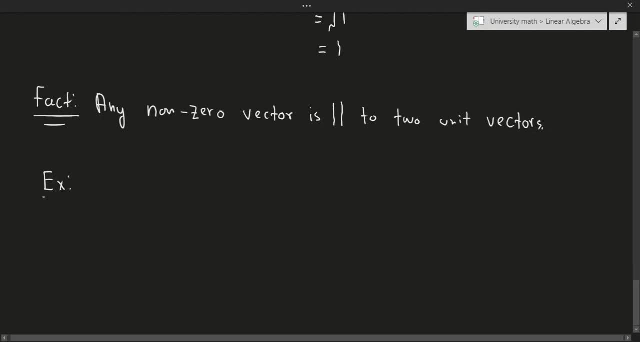 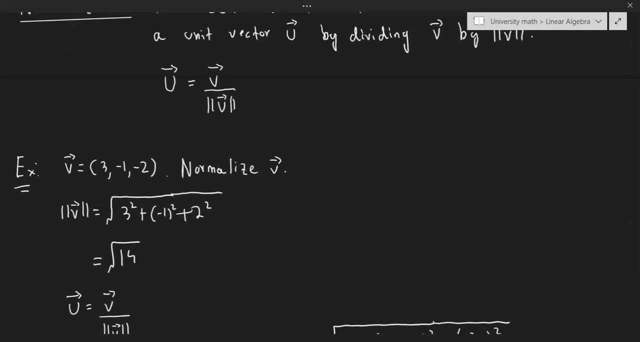 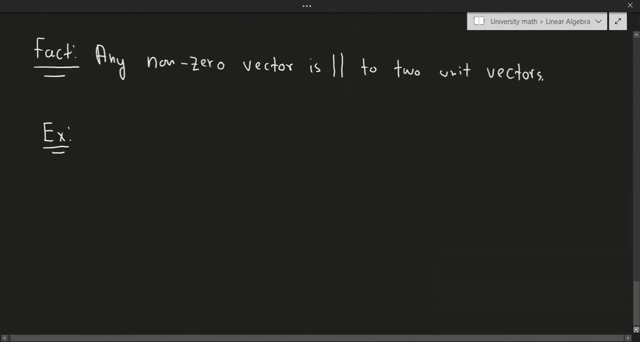 so example: So let's just go back around. So let's just go back around, So let's just go back around up a little bit And let me just go ahead and copy this vector down. Okay, so suppose I give you, v is equal to this vector. okay, So find a unit vector. 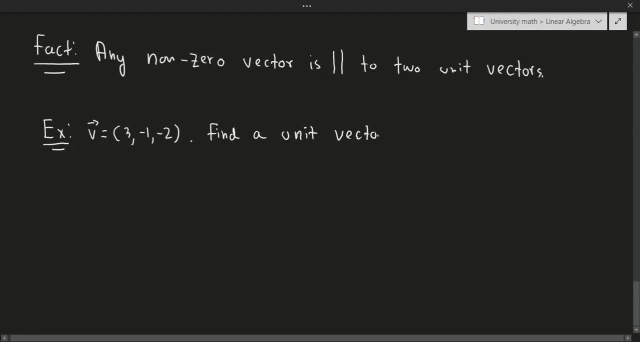 That points in the same direction as v and points in the opposite direction of V. So write that down: So points in the same direction. Hold on, this thing is splitting there. we go Same direction as V and points in the opposite direction as V. 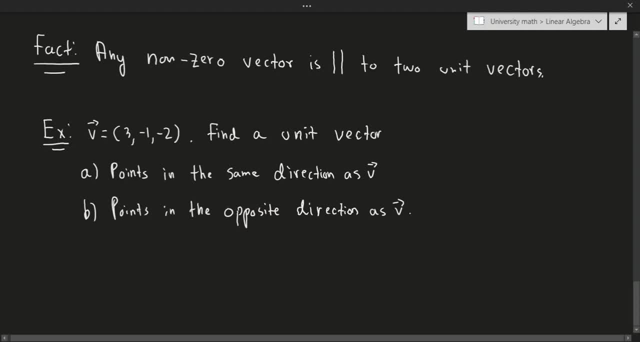 Okay, so essentially any non-zero vector is parallel to two unit vectors, So one of them will be in the same direction and one will be in the other direction. In fact, I'm actually going to write that fact down specifically above. 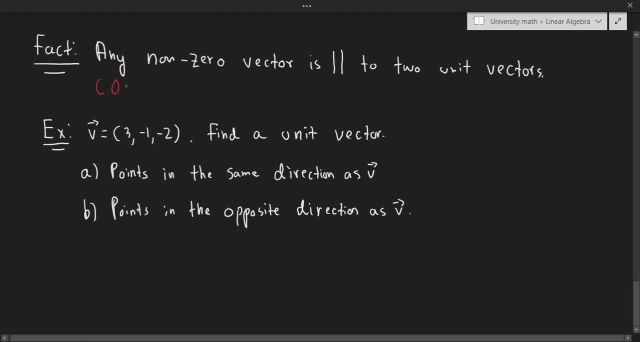 So let me just write that down up here: One in the direction of the unit vector And one in the direction opposite of the unit vector, So one in the opposite, Okay. so that kind of settles this situation here. Okay, so how do we do this? 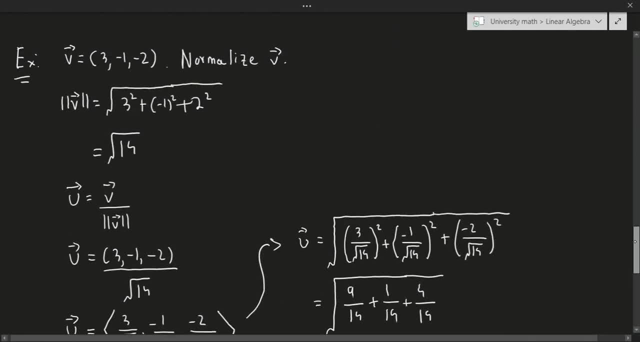 Well, we need the unit vector, and we actually did that already. We found it, Or the magnitude of it. rather, We found that it was equal to the square root of 14.. So let's just go ahead and do that. 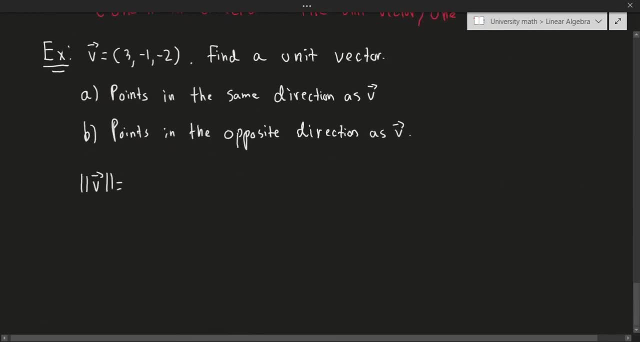 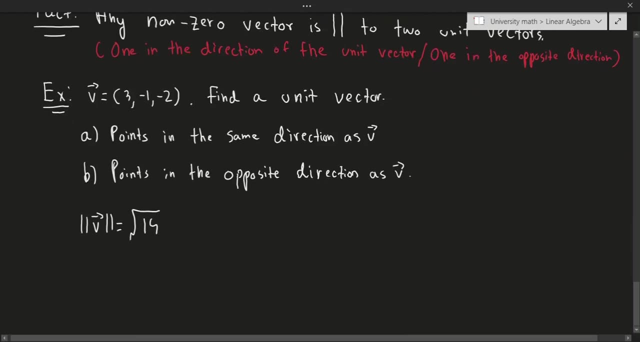 So the magnitude of V was equal to the square root of 14.. We actually did that a little bit above, So in the same direction. well, in this situation, the unit vector: we actually did this question just a moment ago. 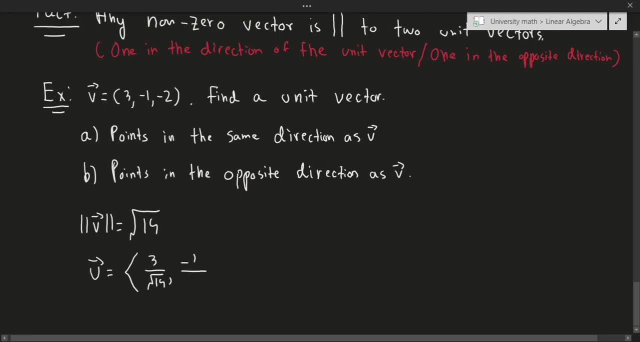 It's going to be 3 over the square root of 14.. Negative 1 over the square root of 14.. And minus 2 over the square root of 14.. Okay, so that's going to be one of the unit vectors. 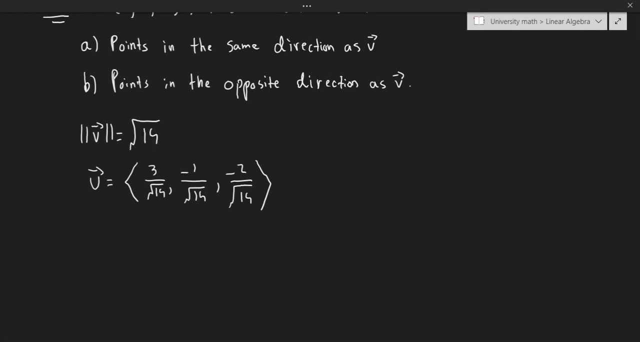 That's going to be in the same direction as the unit vector And the other one is going to be in the opposite direction. So if we want an opposite vector- well recall we talked about this in the previous video- But if we just want to go in the other direction, 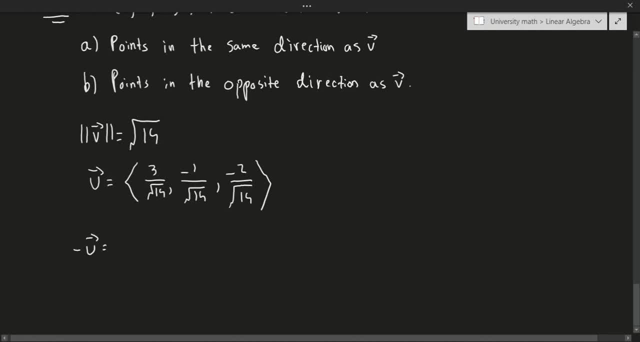 we just take the negative of that original vector. So that's going to give us minus 3 over the square root of 14.. 1 over the square root of 14. And 2 over the square root of 14.. So essentially, our original vector was going this way along, in this direction. 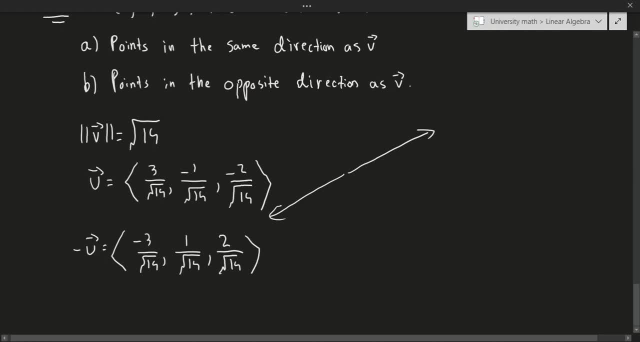 And the other one is just going in this direction instead. So it's the same vector, it's just in a different kind of direction, essentially. Okay, so that takes care of that question. So there's nothing too particularly crazy about this. 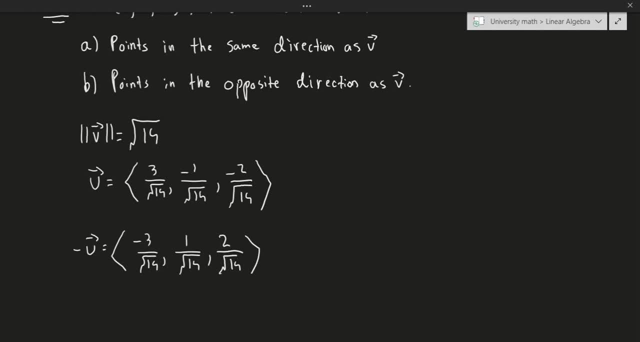 We just have to be a little bit careful about how we use that fact we talked about above. So in the same direction, we just go in the direction of u. In the opposite direction, we just go in the direction of negative u. 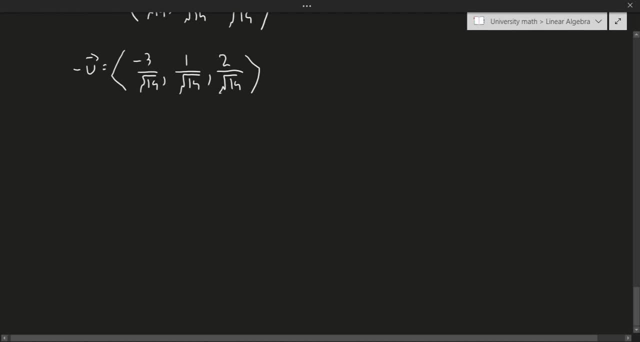 Okay, let's do a few more questions, And this one should be particularly quick. So let's talk about this one And then last one we'll talk about. We'll talk about the concept of a norm a little bit more geometrically. 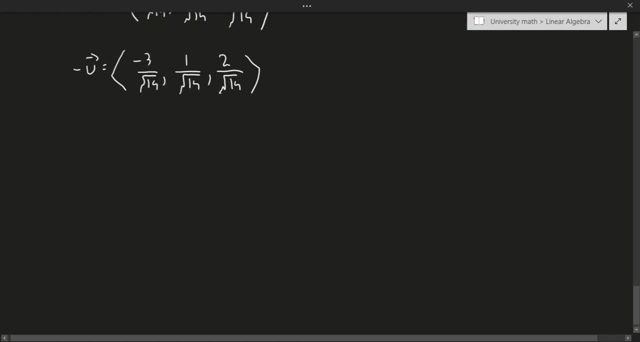 And then that'll be it for this video. So let's talk about the next question. Okay, so let's talk about this one. So consider the points: p is minus 1,, 2, and 4.. And q is 3, minus 1, and 7 in three dimensions. 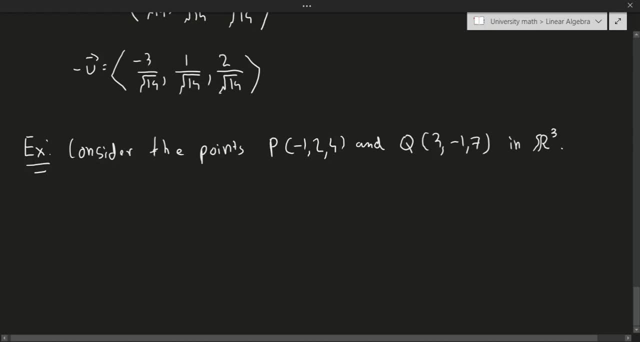 Because we have three sets of coordinates. So we have two sets of coordinates And both of them have three components in each of them. So of course we're in R3.. So find the point on the line segment, And the point on the line segment is a constant. 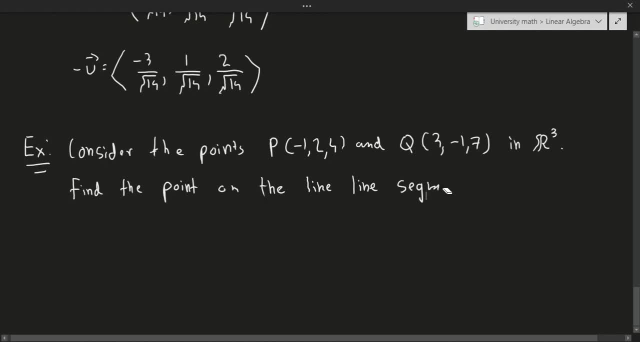 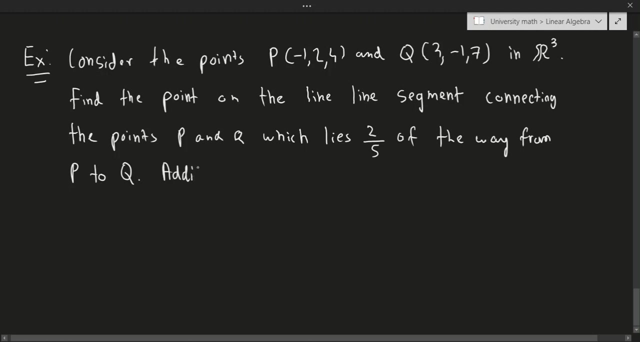 Hold on, Here we go. Okay, so on the line segment connecting the points p and q to the point end of the line segment Which lie, or which lies, rather, two-fifths of the way from P to Q. Okay, additionally, find the magnitude. so let me just fix that writing a little bit. 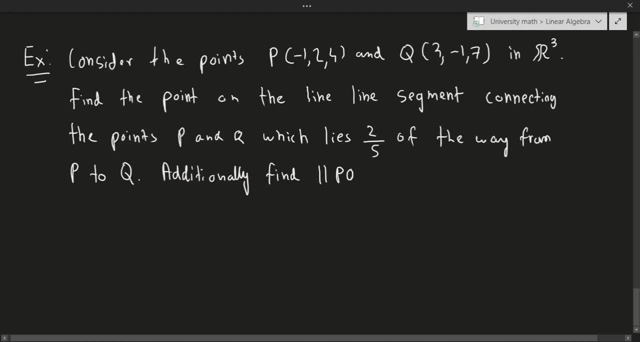 find the magnitude of PQ. Okay. well, if I want to find the magnitude of PQ, well, we just have to go Q minus P and take the magnitude of that vector. So that's simple enough. So the magnitude of PQ is equal to the square root of Q minus P, So it's going to be 3 minus minus 1,. 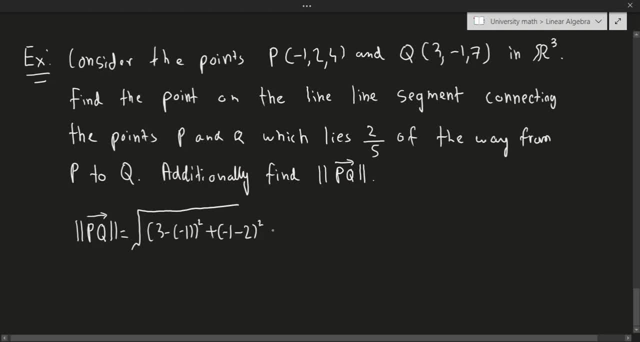 minus 1, minus 2, and then 7 minus 4.. And then, of course, I square each of those components, So that's going to give me the square root of 34.. Okay, so that's the magnitude part done. So how do we do the second part? The second part is a bit. 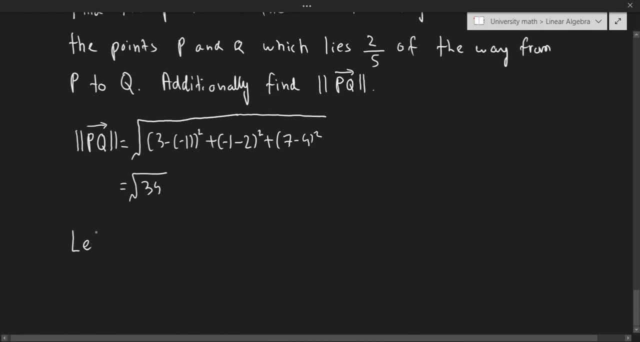 harder. So I'm going to let M be that point which is two-fifths of the way. So let M, which is x, y, z, be two-fifths of the way from PQ. So I'm going to let this arbitrary point 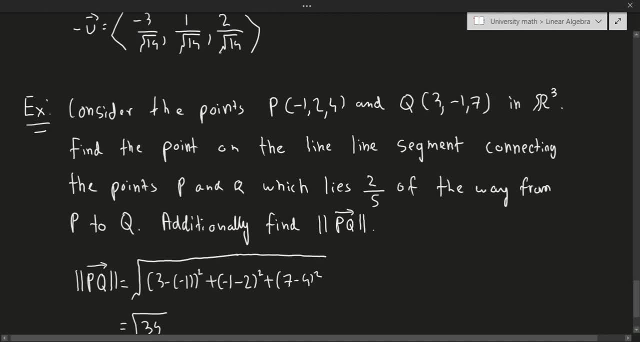 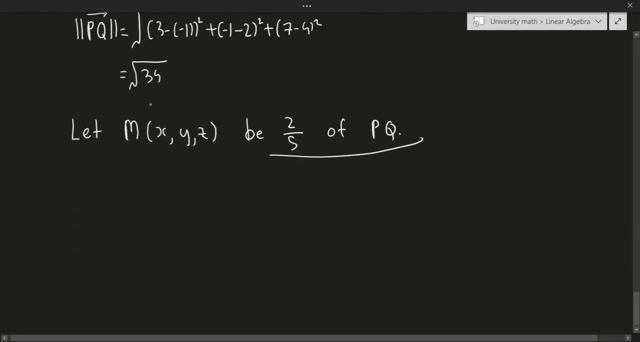 be two-fifths of that particular distance. So find a point which I called M on the line segment. Oh, there's a double line there. That was an accident On the line segment connecting the points PQ, which lies two-fifths of the way from P to Q. So two-fifths of PQ is going to be M. 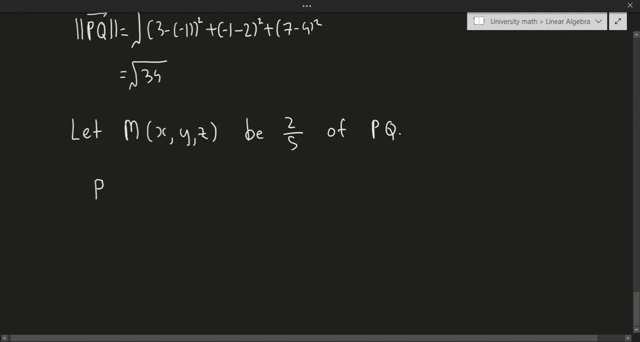 So mathematically, all I'm saying is that PM is equal to two-fifths of the way to PQ. So in a more visual kind of sense, this is essentially what this looks like. So let's go ahead and kind of draw this out. So here's P, here's M and here's Q. So that's P, that's M. 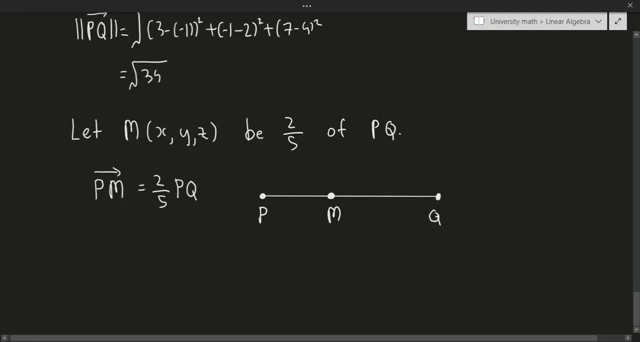 and that's Q. Okay, so this distance right, there is two-fifths of the way from P to Q, So hopefully we can kind of geometrically see what's going on right here. I know that we're in 2D, but let's just pretend that this is kind of 3D. So this point right, there is minus one. 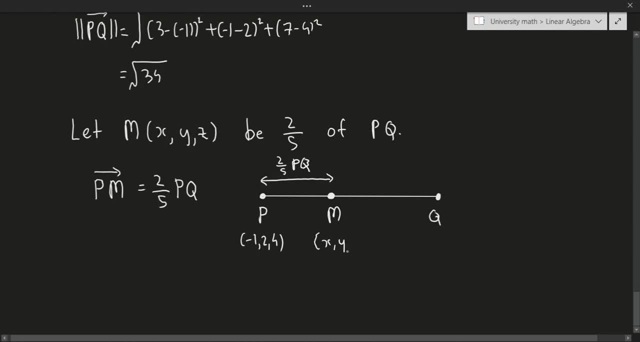 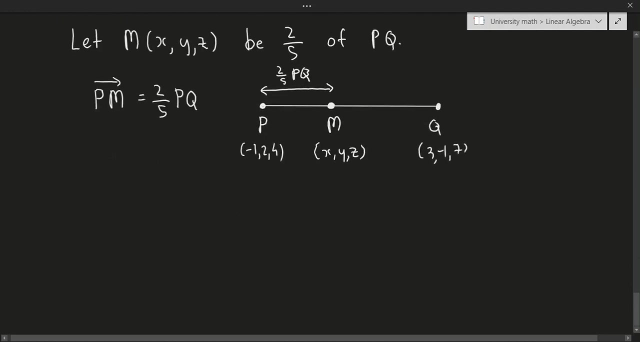 two and four. This point is X, Y, Z And this point right there is three minus one and seven. Okay, so that's kind of the situation that's going on there. So the distance from P to M. 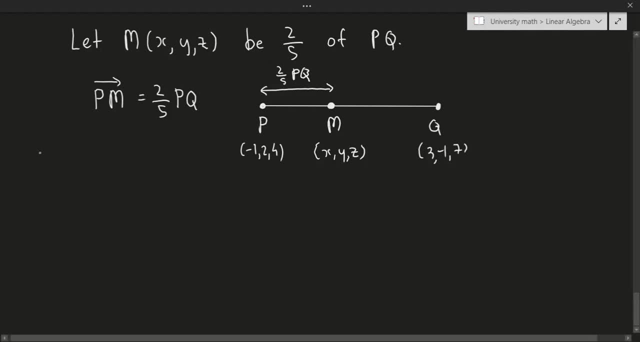 well, that's M Minus P. So essentially what we're going to get is X plus one, Y minus two. Z minus four is equal to two-fifths of the way from P to Q. So Q minus P, so that's three minus minus one, So that's four. 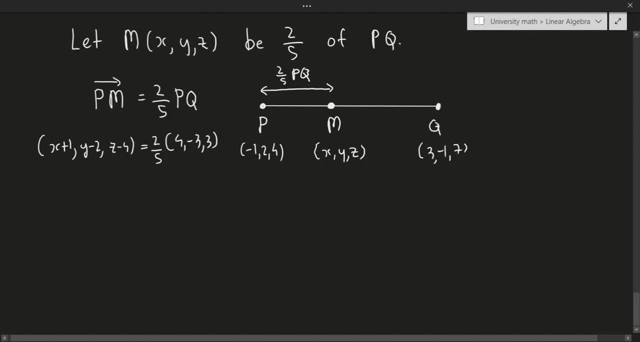 minus three and three. Okay. so if I kind of compare these components term by term, we're going to get: X plus one is equal to eight over five, Y minus two is equal to minus six over five And Z minus four is equal to. 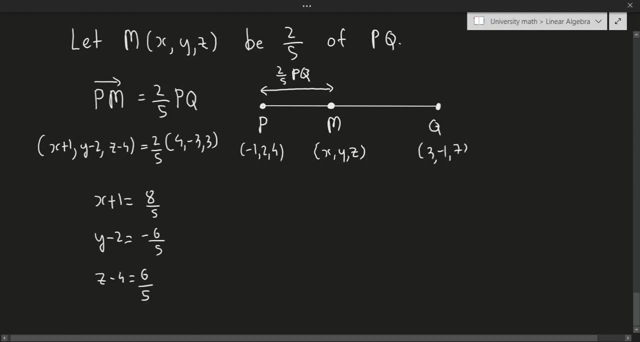 six over five. So as a result, we can directly solve for each of these components and we get that X, Y and Z respectively are equal to three over five, four over five, 26 over five. So this will be: 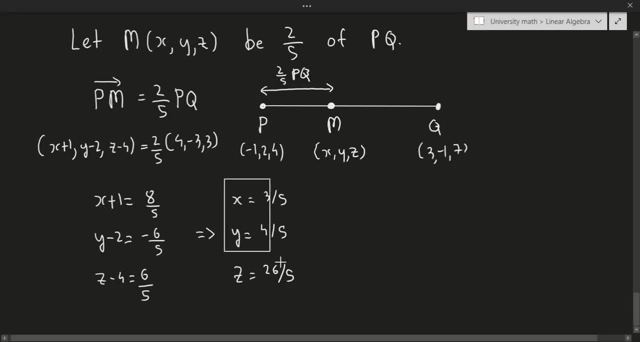 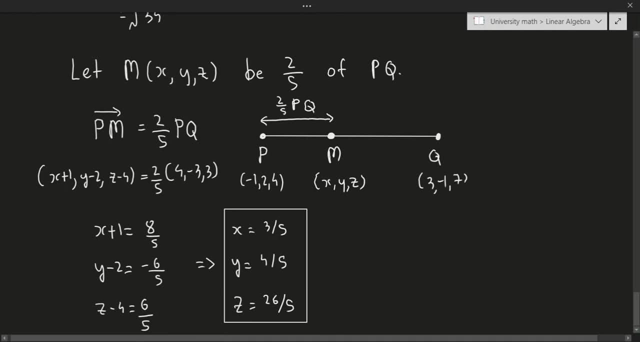 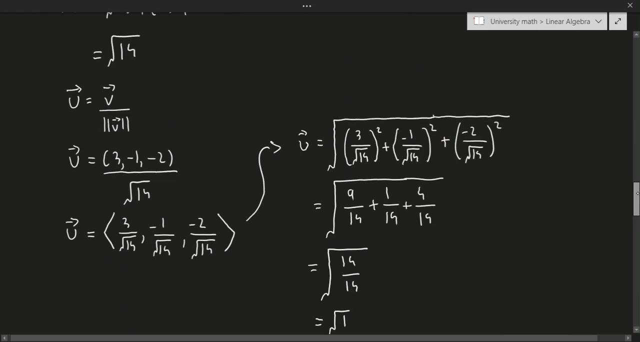 the point that is, two-fifths of the way from P to Q, And we're done, So hopefully that made sense Intuitively. this should make sense from the drawing, but if it doesn't, feel free to leave something in the comments and I'll be happy to answer Now. we have more or less finished. 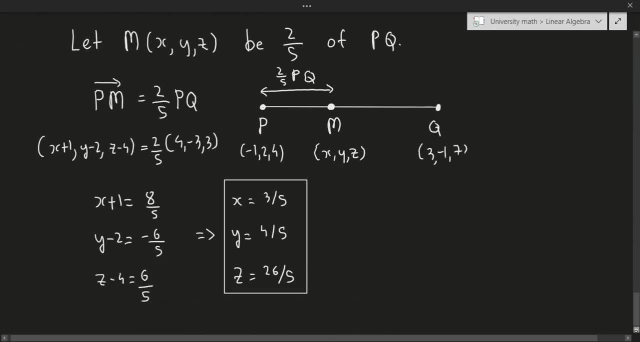 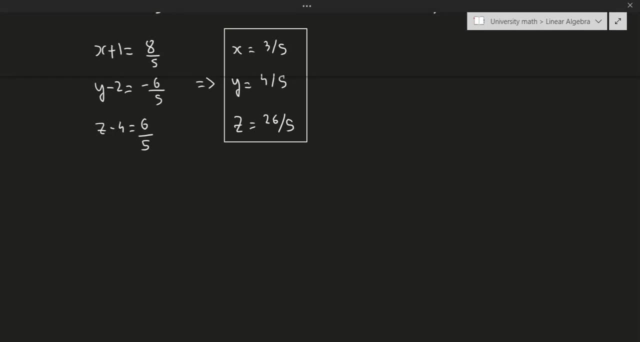 everything. Now there's one last thing I want to talk about, and that's kind of the geometric interpretation of norm. This one is a very short section, so we don't have to do too much here. Essentially all I'm saying. 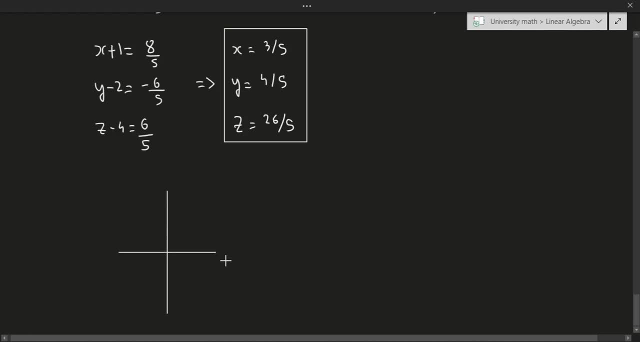 is that we can interpret the idea of a norm by simply just considering the Pythagorean theorem of some kind. So let me just go ahead and draw a triangle And, to be very clear, I'm actually going to erase this thing and draw a right-angled triangle. 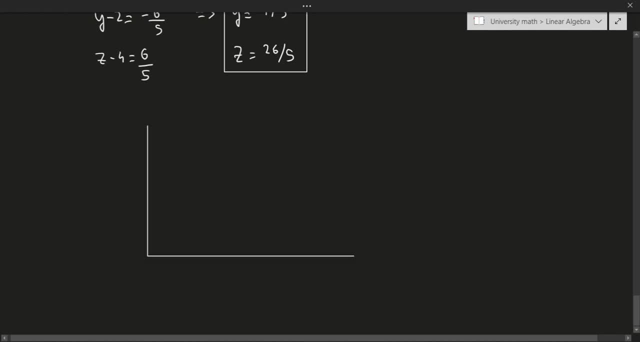 using a much shorter kind of axis like that. Okay, so let's just draw a triangle And here we go. Okay, and let's just go ahead and draw a line going down. That's going to go from here, And let's see, that's going to go here. 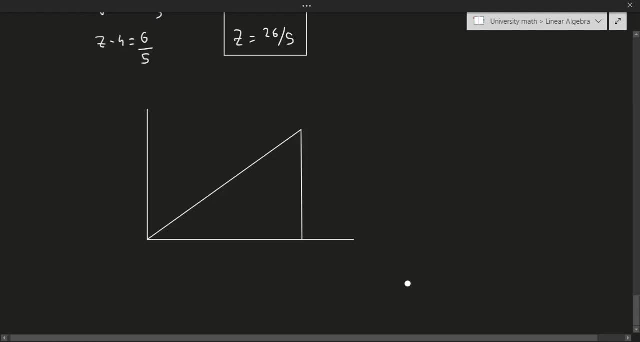 Okay, so let's call this vector right here. Oops, I just undo that. Give me a second. Okay, let's call this distance from here to here. let's call that v1.. Let's call this distance v2.. So, by the definition of the Pythagorean theorem, this distance right there. 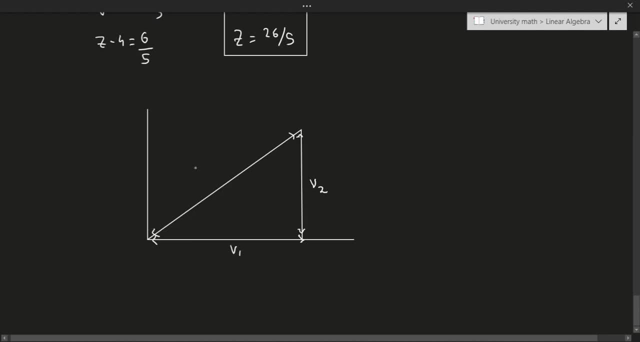 the hypotenuse of this triangle is the square root of v1 squared plus v2 squared, But by definition that is the norm. So the magnitude of v is the square root of v1 squared plus v2 squared. So you can think of the idea of a norm as a n-dimensional Pythagorean theorem. 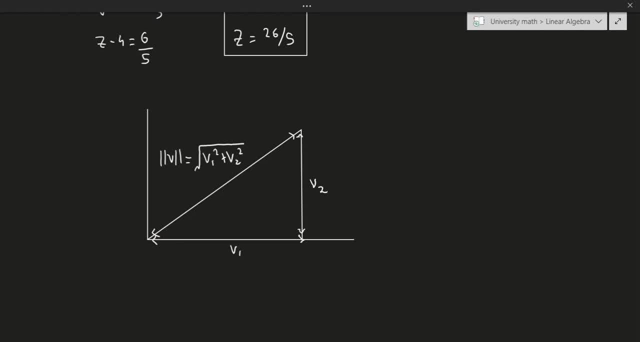 Of course, in three dimensions we'd use three components. In four dimensions, we'd use four components, and so on and so on. So you can think of the idea of a norm as a n-dimensional Pythagorean theorem. This isn't necessarily 100% accurate, but you can kind of interpret this. 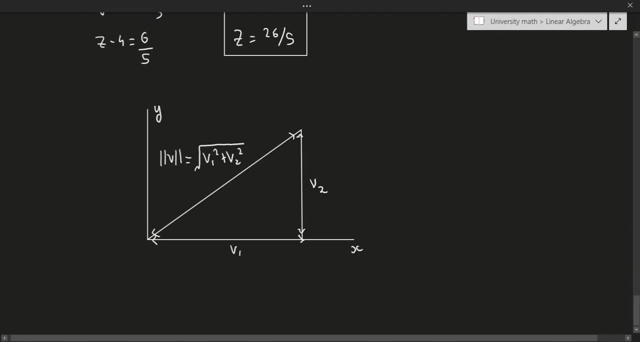 geometrically this way, at least the idea of a norm. So this is how you kind of interpret this, And aside from that, we have now more or less finished the idea of norm. So that card, that is it for this video. 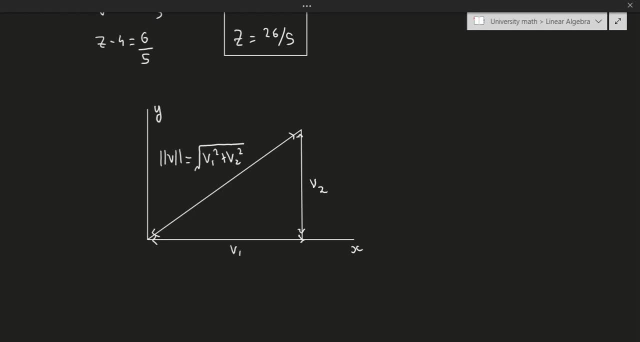 So if you have any questions, feel free to comment your question and I'll be happy to answer as soon as I can. But otherwise, if this video helped you, please remember to like, comment, share and subscribe. We're almost at 900 subscribers and almost 1000, so I'm very excited to achieve that milestone. 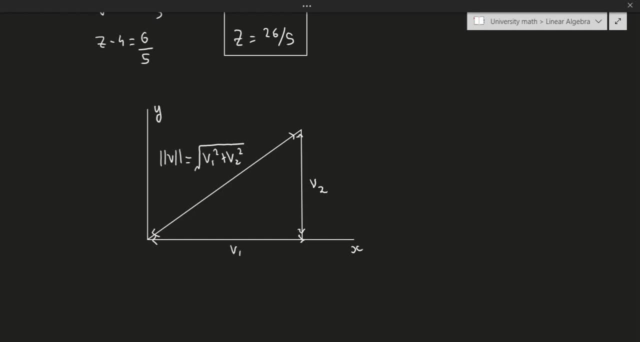 So if you could please share my video around and my channel around, that would be greatly appreciated. So I will see you all in the next video. Have a great day.